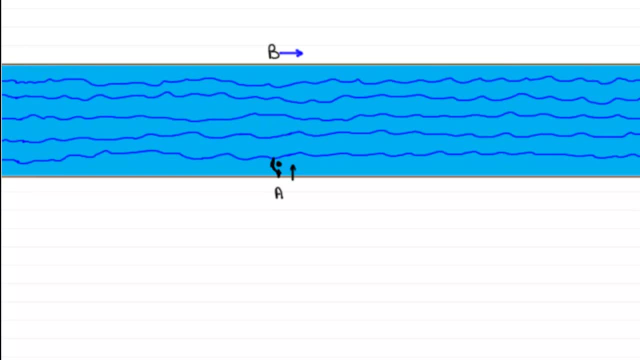 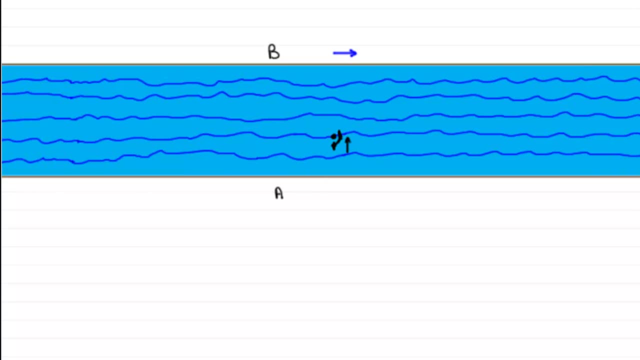 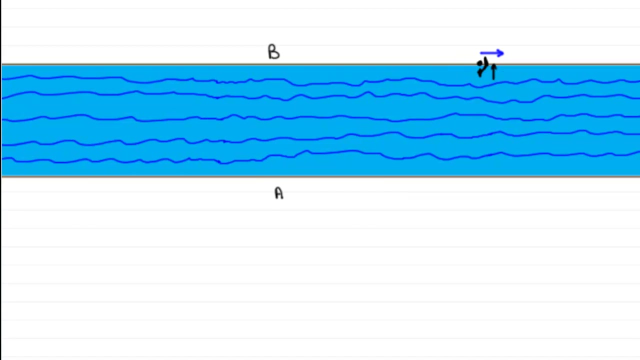 Well, that is the aim of this video. So if the swimmer decides to swim from A to B and there is a current in the river, then what happens is that he gets carried downstream. So why is this? Well, if we look at the swimmer's velocity when he is swimming in still water, 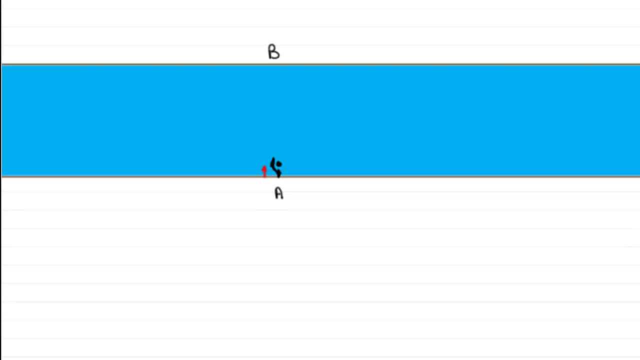 illustrated by this red vector. we saw earlier that he had no problem swimming across the river river from A to B in still water, but then when we had the current moving from left to right illustrated by this blue vector, then when the swimmer wanted to, 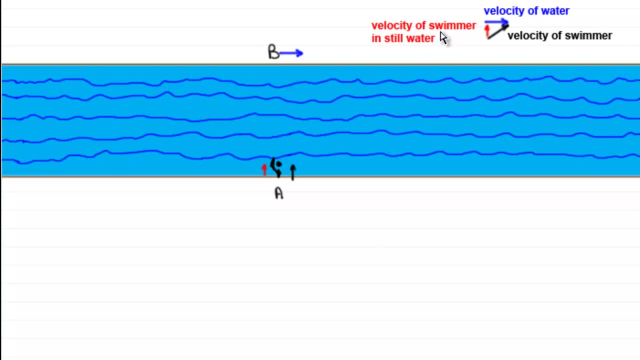 swim across the river. the velocity of the swimmer in still water illustrated by the red vector, combined with the velocity of the water illustrated by the blue vector, resulted in this swimmer swimming at this angle here with this velocity. Let's just run that through again so we can see now at that as the 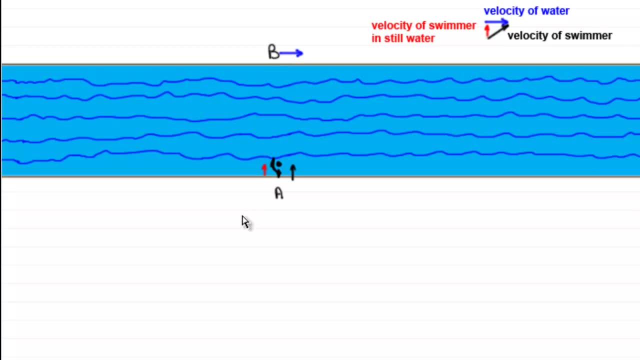 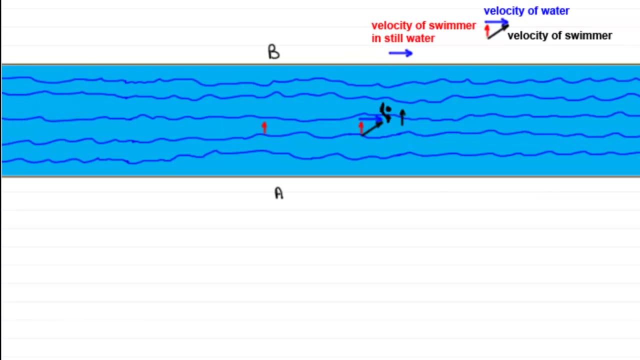 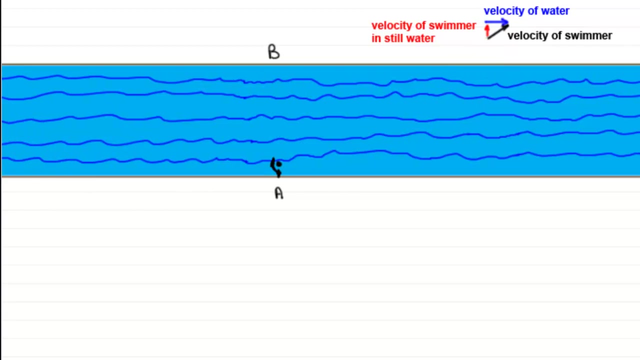 swimmer starts off heading towards B, then the combination of those two vectors makes him go at this diagonal course downwards stream. now suppose the swimmer wants to swim from A to B, how's he got to go? but he's got to head upstream, he's got to aim upstream, and if this is his, 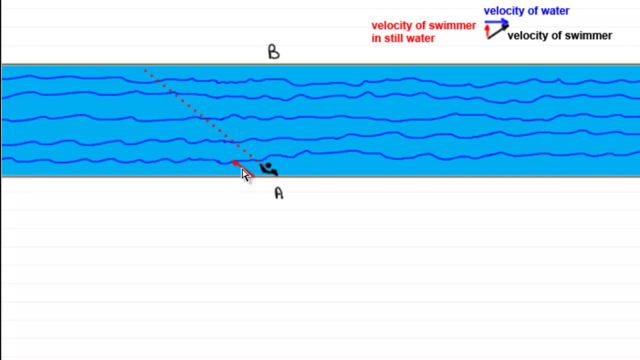 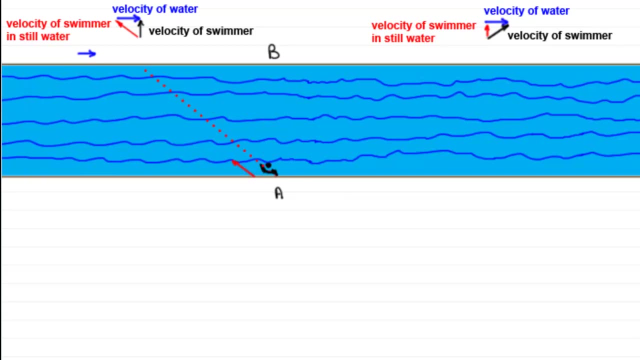 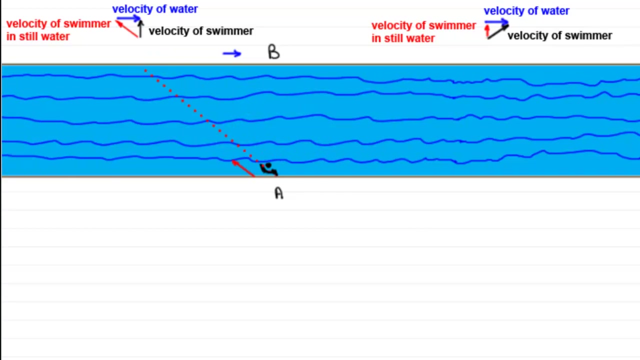 velocity in still water if there was no current, then if we look at combining the vectors of the water, the velocity of the water with the velocity of the swimmer in still water, we would get an effect where the swimmer can swim directly across the river, providing he can swim hard enough to overcome the velocity of. 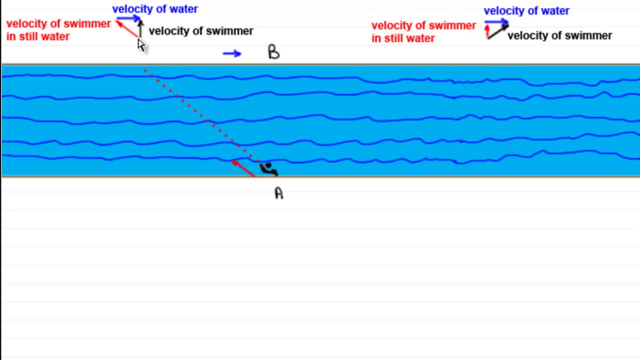 the water. the combination of his swimming in still water with the velocity of the water results in the velocity of the swimmer heading across from A to B. let's have a look, see how that happens, so you can see that that combination there allows the swimmer to. 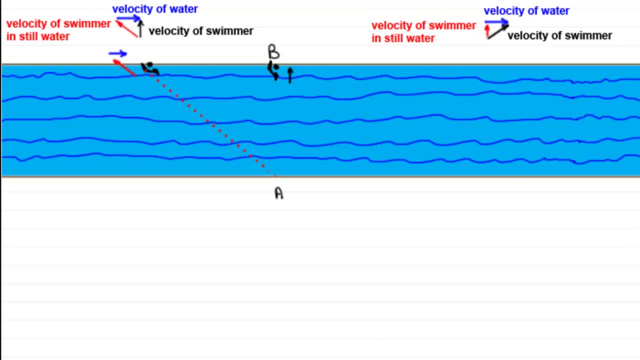 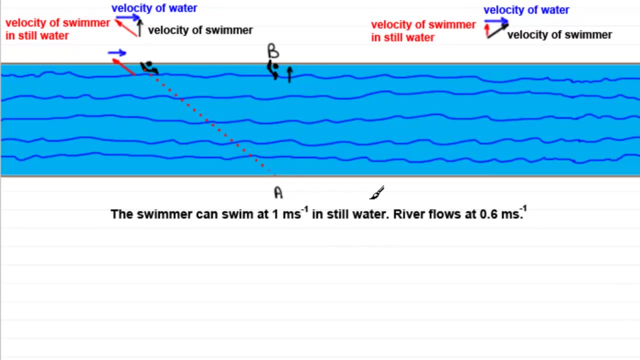 swim from A to B. now let's just do a few calculations. let's suppose that the swimmer can swim at one meter per second in still water and the river flows at naught point six meters per second. then let's work out the velocity of the. 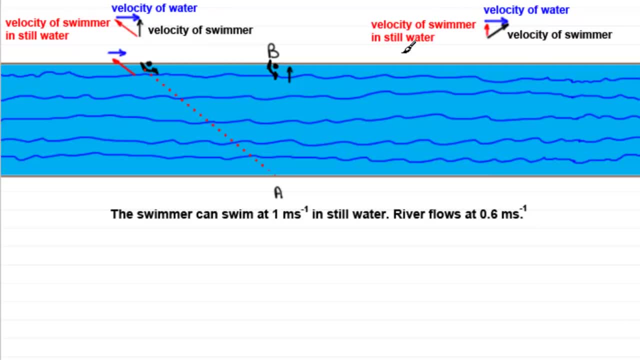 swimmer in each of these scenarios- and we'll start off with this one here- and so, if we're drawing the vector triangle, we start then with the velocity of the swimmer, which we mark in as a velocity vector- one meter per second, going straight across the river in the direction A to B, and then we've got the 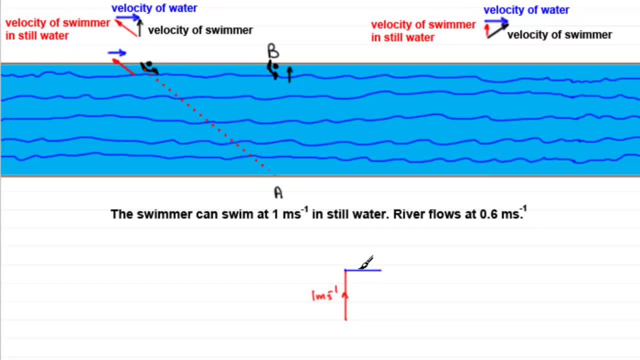 velocity of the water left to right here, going at naught point, six meters per second, and then the resultant velocity of the swimmer in indicated by this black vector. we'll call it V. so how are we going to work out V? well, that's easy, because all we need to use is Pythagoras' theorem. 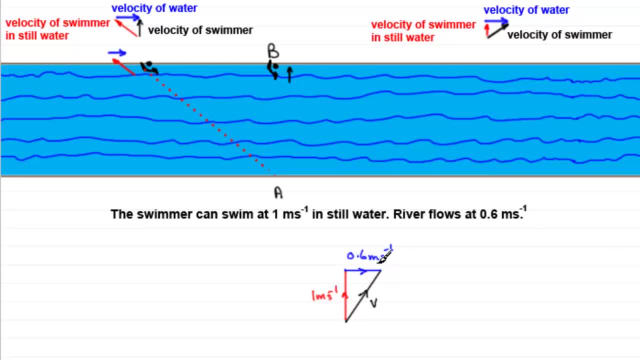 remember, V squared will equal 1 squared plus 0.6 squared, because it's a right angle triangle. and so to work out V, then we just take the square root of 1 squared plus 0.6 squared and if you work that out you'll find that you end up with 1.166, and so on. 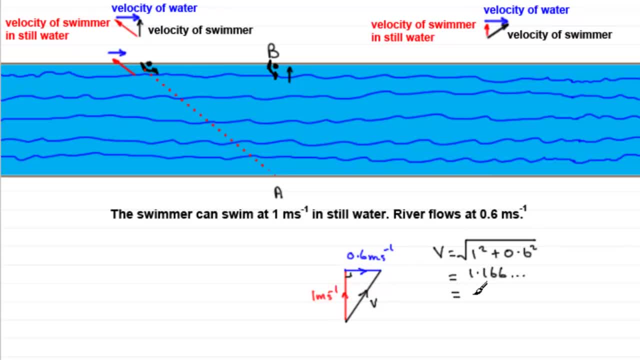 and if we round that, say, to one decimal place, that would be 1.2 meters per second. and when it comes to the angle, say the angle made with the direction AB, we'll call that angle, say theta. then what would theta be? well, we can do that from. 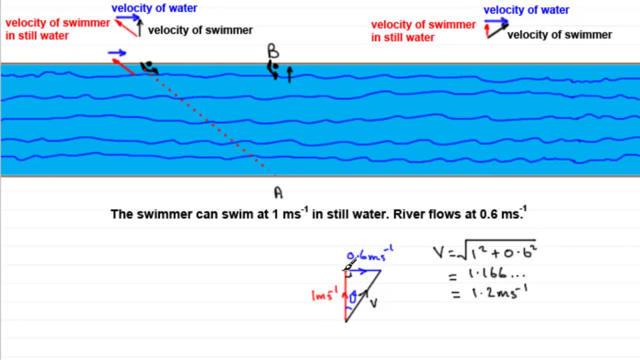 trigonometry, this would be the opposite side. this would be the adjacent side to theta, so it would be tan. theta equals 0.6 over 1, and so theta would be then the inverse tan of 0.6 divided by 1, and if you work that one out, you end up. 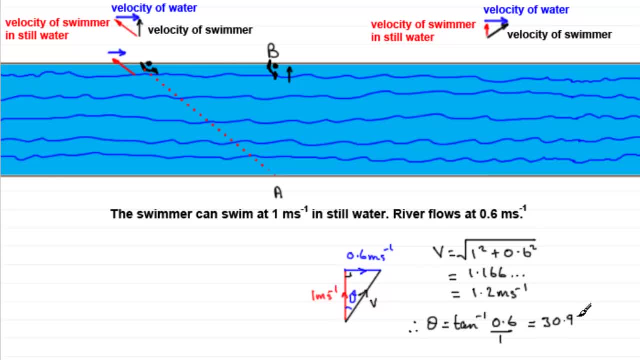 with 30.963 and so on, degrees. if you round that, say, to one decimal place, you're going to get 31.963, greater than the value of zero to 1.9 when remove those and you're going to get 32.9, and by that that's cuts the. 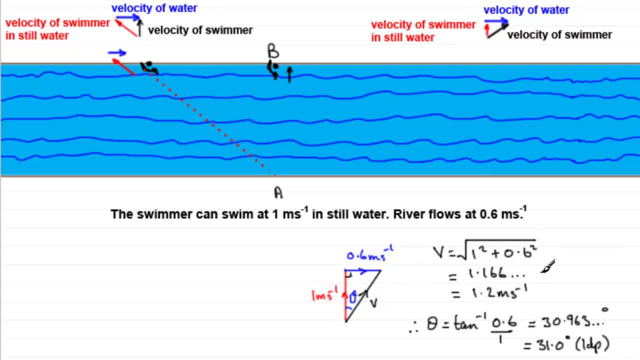 Display component in the dialog box the value. sorry, thanks for watching. if you like this video, then you're not watching the video for the encyclopedia today, everybody. no, we got reality on it. K the matter to us catches Tom. let's just draw it in again. we'll put in the velocity of the swimmer in still. 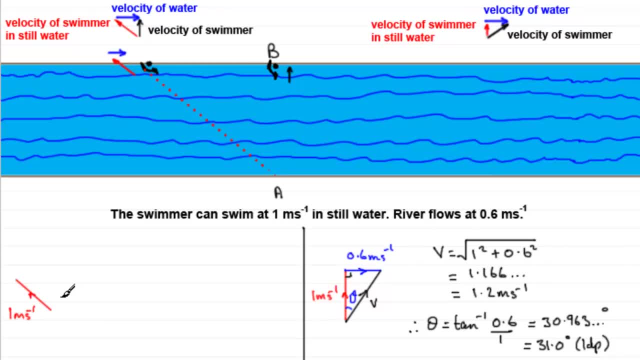 water. that's one meter per second. we've got the current bringing the swimmer back on course, going from A to B. this is nought point. six meters per second, and you've got the resultant velocity then of the swimmer. call it V, so to get V. 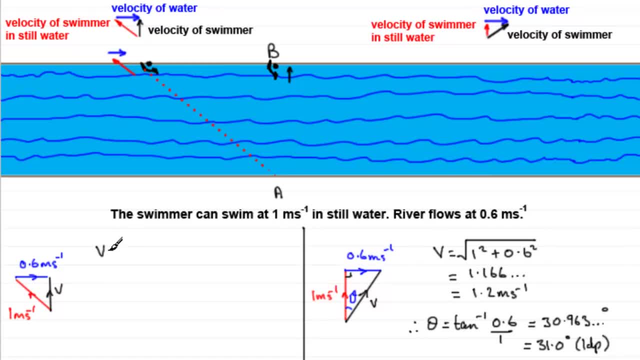 again, all we need to do is Pythagoras theorem, but remember, this time this is a shorter side in this right angle triangle, so it will be: V squared will equal one squared minus nought point six squared. so we end up taking the square root of that. so V equals one squared minus nought point six squared. and if 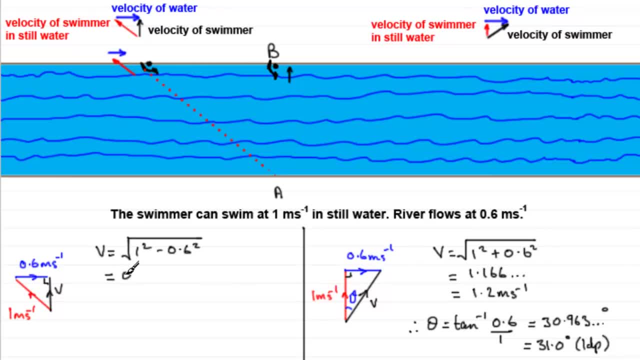 you do that, you'll find you get exactly nought point eight, nought point eight meters per second. and for the angle that the swimmer has to take, this to say it's this angle in here will call it alpha, then twerk out alpha basic trigonometry here. now that we know all three sides, you could use any. 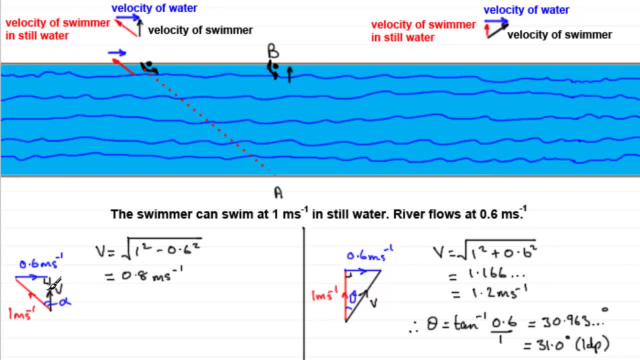 trigonometric relationship sine cos or tan, but I'm going to go for sign in this particular one, just purely because I was given these two sides. so sign of Alpha equals opposite over hypotenuse 0.6 over 1, so therefore alpha must be equal to the inverse sine of 0.6 over 1.. 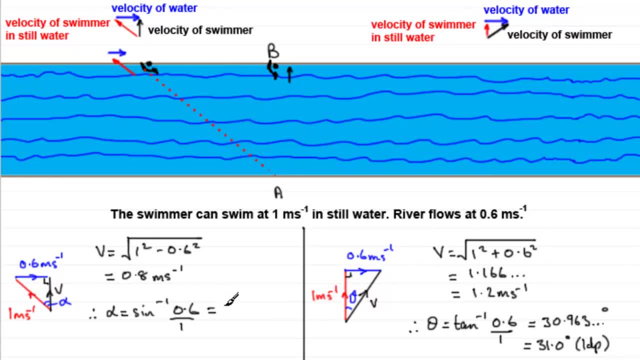 And if you work that out, you end up with 36.869 and so on degrees, And if we round that to say one decimal place, it's going to be 36.9 degrees to 1 dp. Okay, so I hope that's given you some idea, then, how you can handle problems of this particular type.